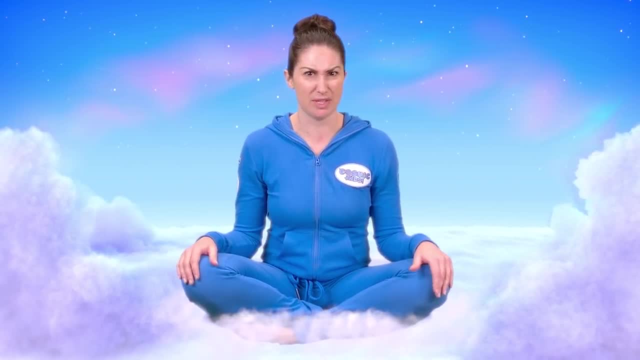 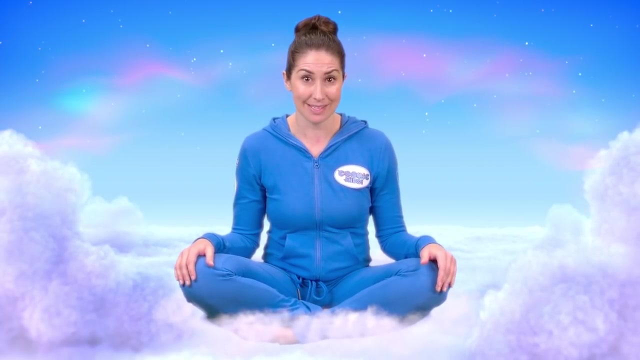 dad. You have no idea why, because it wasn't your fault, But they say something mean to you and it makes you feel really angry and maybe a bit sad too. Afterwards you might find yourself going and doing something mean to someone else Like: how do you feel about? 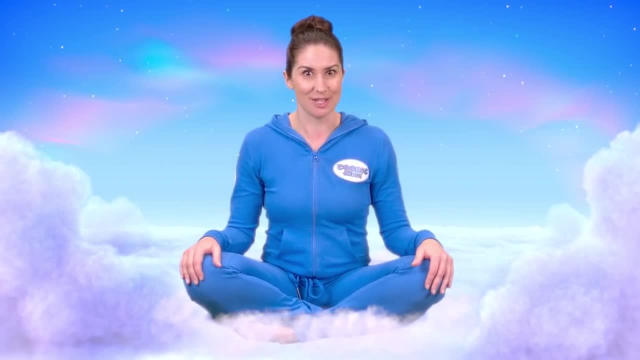 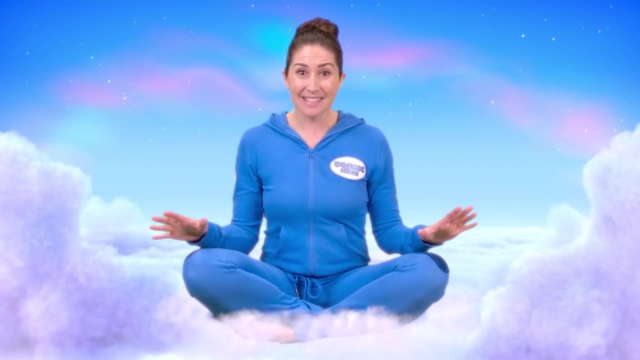 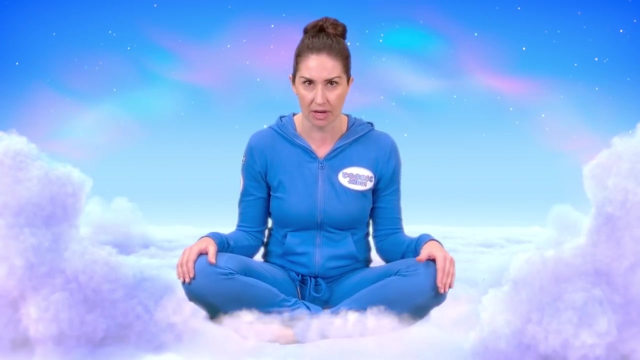 that, Or reminding your brother or sister's favourite toy because you know how much it annoys them. Or reminding them of how bad they are at maths. Or telling someone at school that it's fish and broccoli for lunch, when you know how much they don't like fish and broccoli. 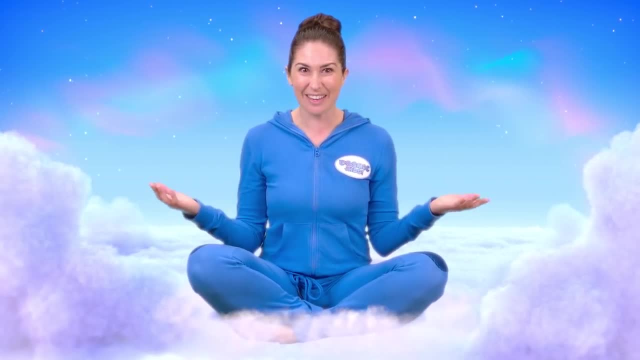 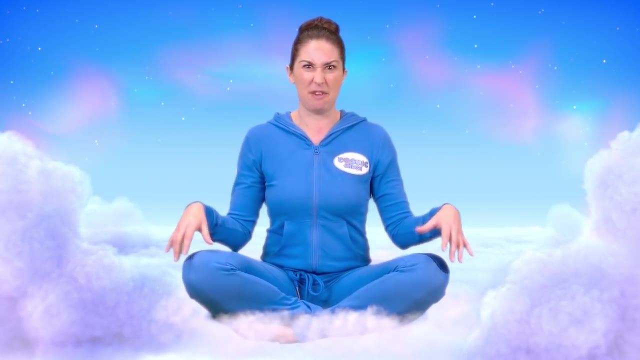 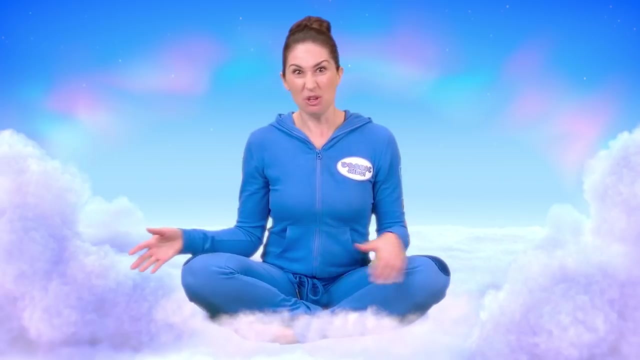 This is why people are mean. It's like a bug, The mean bug. Someone is mean to you and it makes you feel: yuck, You've caught their mean bug. To get rid of the mean bug, yuck, you chuck it at someone else by being mean to them, So they get landed with the mean. 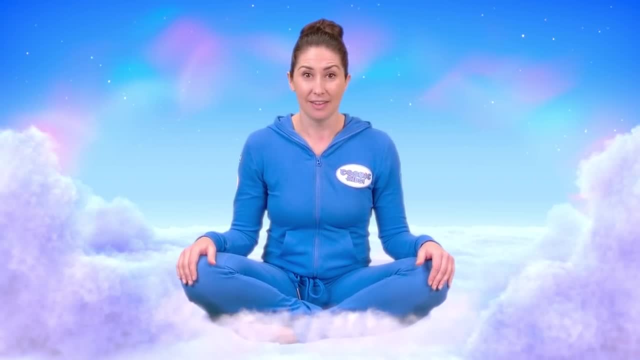 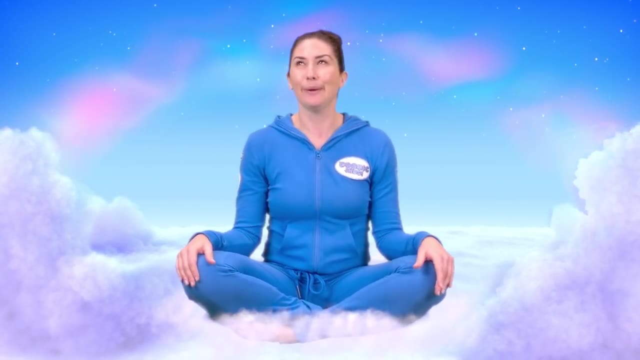 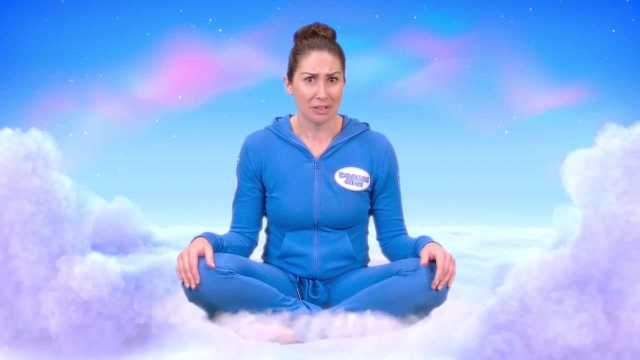 bug yuck, and it just keeps going. After that, for a little while it feels better. Phew, I'm glad I got rid of my mean bug, All that yucky feeling. But unfortunately it doesn't work as easily as this, Because the mean bug loves it when 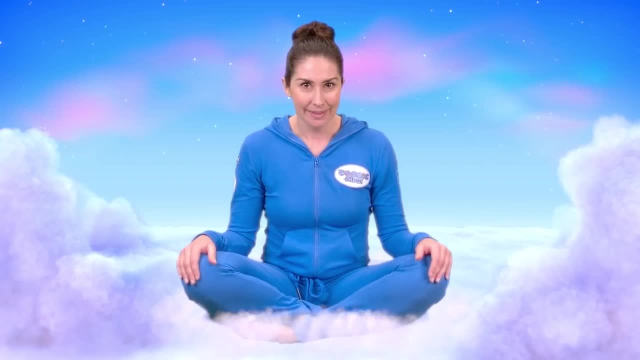 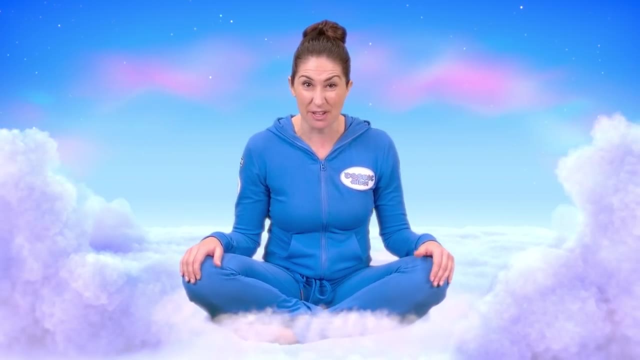 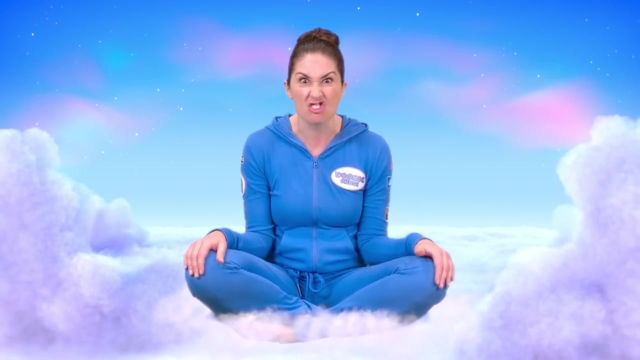 you are mean And will pop up again After feeling better. you might start to feel bad for being mean. You might have a bad dream about it Or go round with a moody, grumpy, snarly frown face, feeling a bit grrrrr. You might be thinking that some people are. 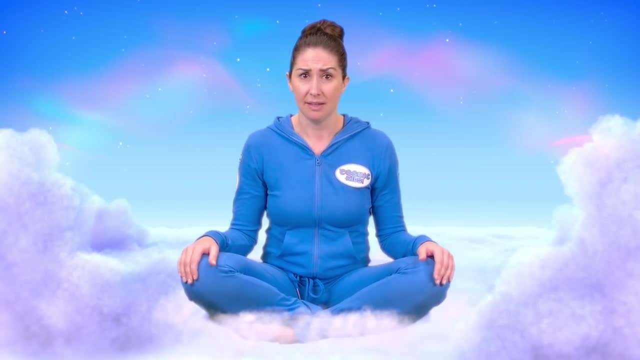 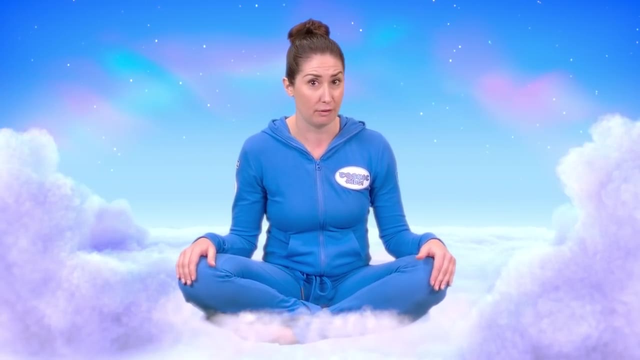 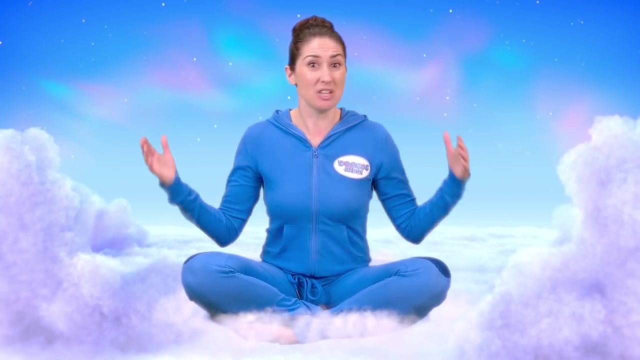 mean. But because they are mean to everyone, you can be sure that no-one will like them very much And they probably won't have any friends, Which makes them even more sad and angry, Which makes the mean bug in them get even worse.